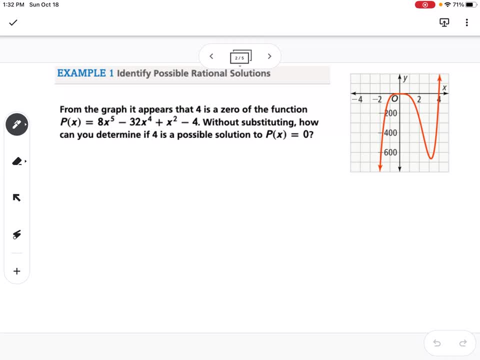 So we're using it kind of as a first step to check stuff. So our possible rational zeros we call p over q, And so your p values are going to be factors of the constant And your q values are going to be factors of your leading coefficient. 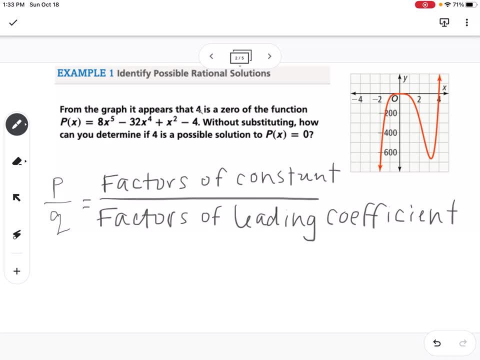 Okay, so factors of the constant in this case. So your constant is negative 4.. So when we list out the factors of the constant, we have to say we know that negative 1 times 4 is a factor, as well as one times negative four. 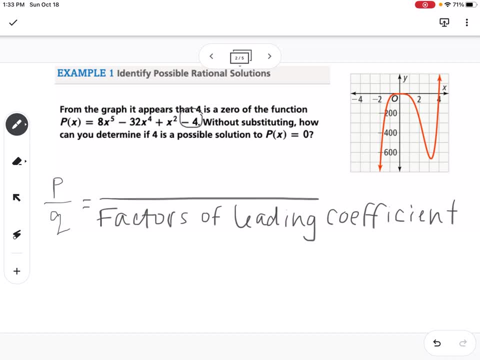 So the negative could be either way. So the way that we list these is we always put a plus and minus in front of each one. So my factors of four are one, two. I kind of like to go up the like, start with one and go all the way up to the number. 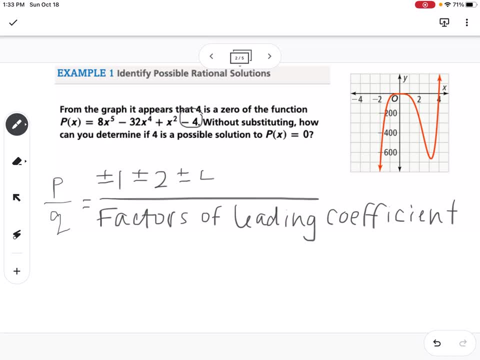 So one is a factor, two is a factor, and then four is a factor. So those are all my factors of four. So then the denominator is the factors of the leading coefficient. So the leading coefficient in this problem is eight. So our factors of eight are one, two, four and eight. 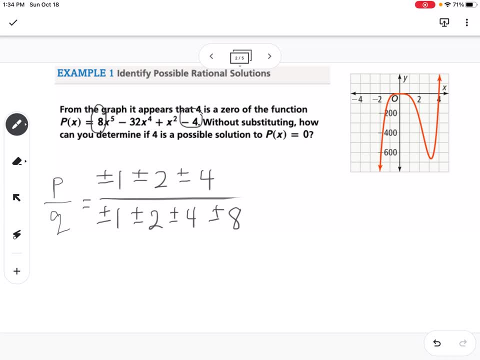 So when you're doing a big, long problem, it's okay to leave it like this if it's part of the overall problem. But if you're asked to find the possible rational solutions or possible rational zeros, you wanna actually take the time to divide this out. 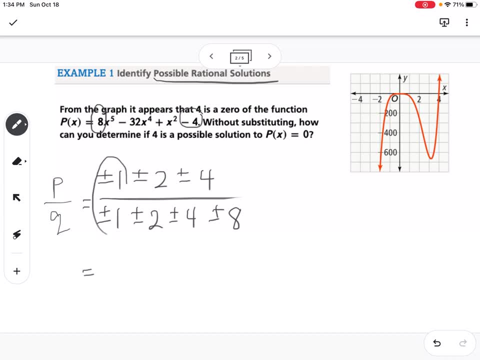 So this would be: we're gonna write the, we're gonna write the actual list. So if I take one divided by one, I get one. If I take one divided by two, I get one half. If I take one divided by four, I get one fourth. 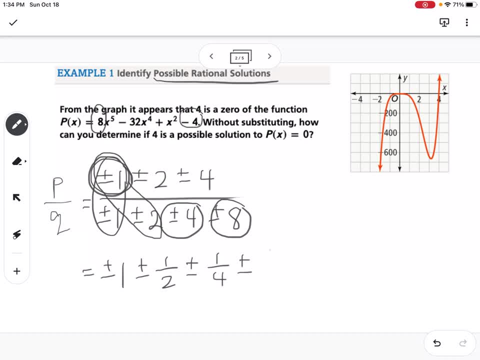 And one divided by eight, and I get one eighth. Now, as I go on to the next numbers, if I already have the number in my list, then I don't need to write it again. So if I take two divided by one, 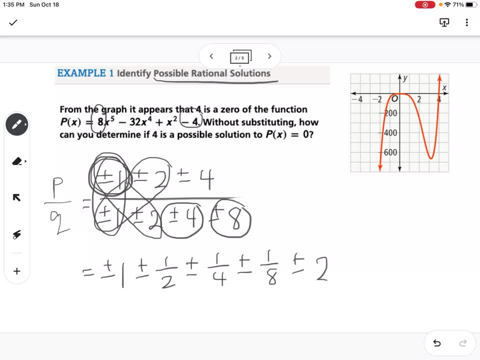 that's two. Two over two is one, and I already have that in my list. Two over four is one half- I already have that. And two over eight is one fourth, which I already have. So then I'm gonna take four over one is four. 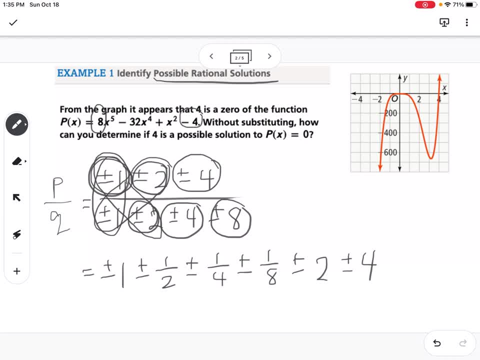 And four over two is two. I already have that. Four over four is one. Four over eight is one half, and I already have that. So this right here I'm gonna take four over one and that right here is my list. 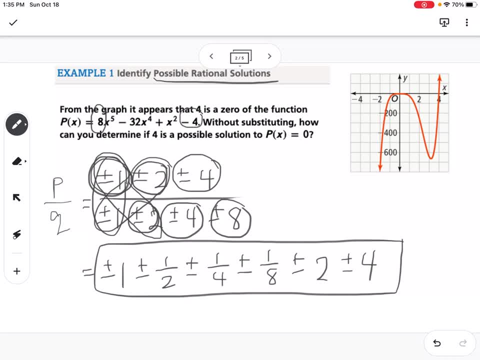 So those are all my possible rational zeros. So if you look at the graph, we can see that four is one of the zeros here and we can notice that four is in my list. So that's why a possible rational zero list can be helpful. 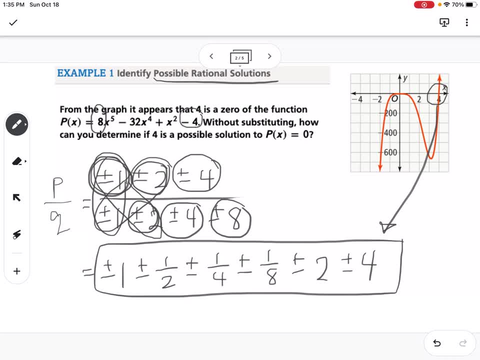 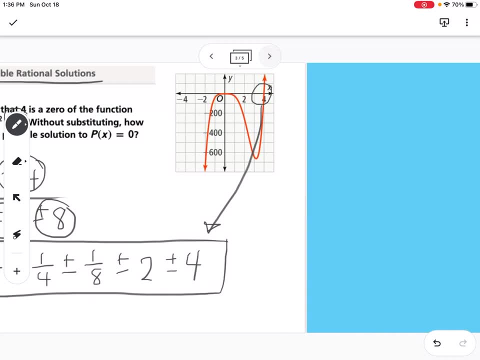 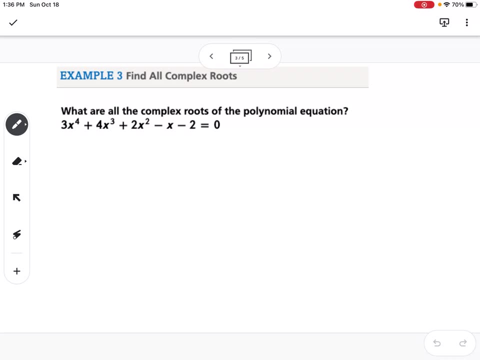 because you can use it to determine where the graph is crossing the x-axis without actually having to find the zero. Okay, So our next example is to find all complex roots of the polynomial equation. okay, We're going to find all the zeros. 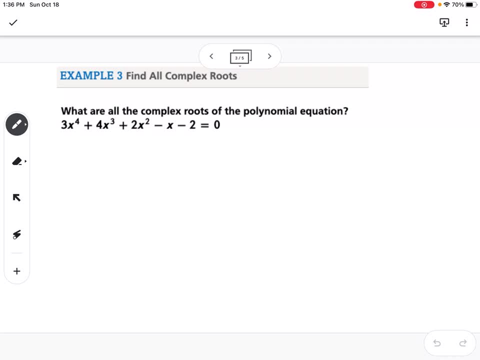 So the process I would like you to practice when you're going through these types of problems is: step one is to do a p over q list. Step two is to graph and use the graph and your p over q list to determine where it looks like your graph is crossing. 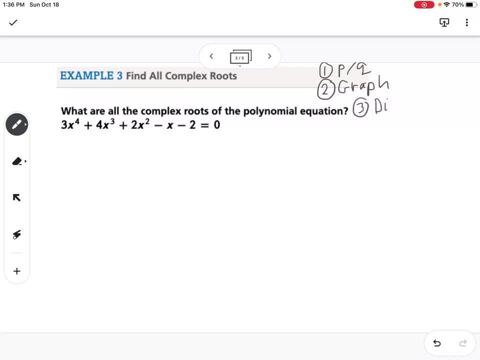 And then three: you're going to use division, so synthetic division, to narrow down, get your function simplified, And then the last step might be to factor. It might be to use the quadratic formula. It kind of depends on what you're left with, okay. 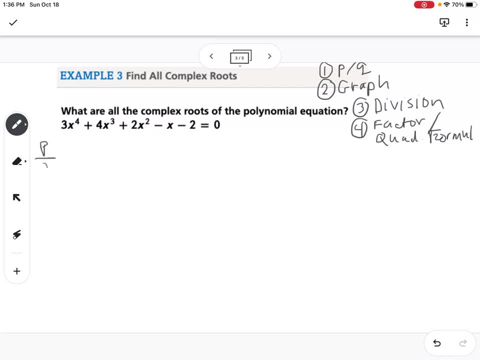 So we're going to use this as an example. So the first one: The first thing I'm going to do is make my p over q list. So my constant in this case is 2, so my factors are 1 and 2, and my leading coefficient's. 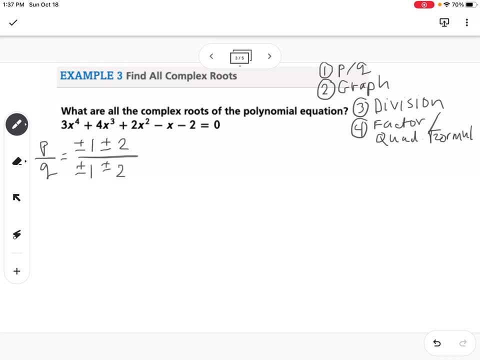 3.. So that's 1, 2, no 1, 2, 1 and 3, okay. So that means that my possible rational zeros would be 1, 1 third, 2, and 2 thirds okay. 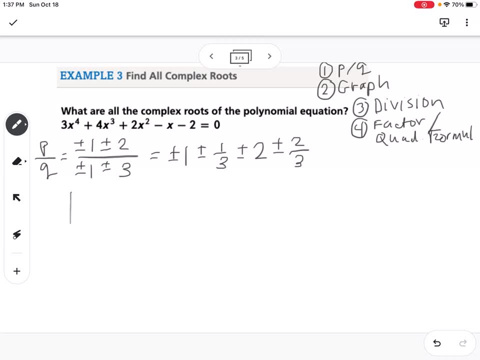 So then I'm going to go to my graph And I'm going to graph it, And if we graph it, what it looks like is not quite a quadratic, but it looks like it's crossing in two spots. So this is where your p over q list can be helpful. 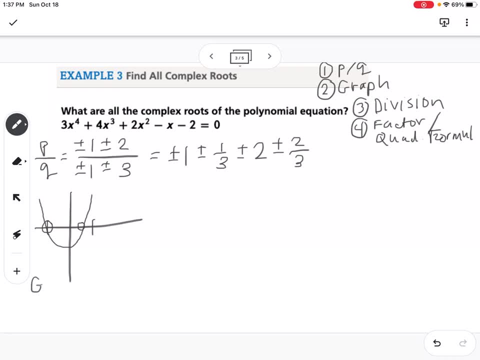 So if you're looking at the graph, it looks likeso. from the graph, it looks like it crosses at negative 1. Which is on our graph, On our list, So that's good. And it also looks like it's crossing- not quite at positive 1.. 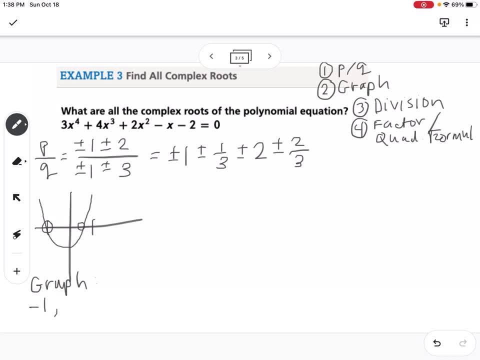 So if I look over at my list, I think: okay, what number, which value is not quite positive? 1? And I could say positive 2 thirds. So I'm going to check these using synthetic division now. So my first one. so I have 3,, 4, 2, negative 1, negative 2.. 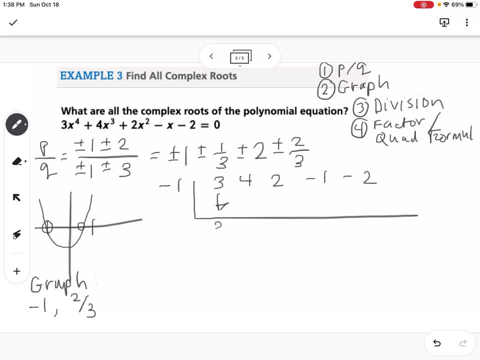 And I'm going to check negative 1. And it works And it worked. So now here's the nice thing: If you have a remainder of zero, rather than re-go back to your original function, you can take this solution now. this simplified: this would be 3x to the third power and we. 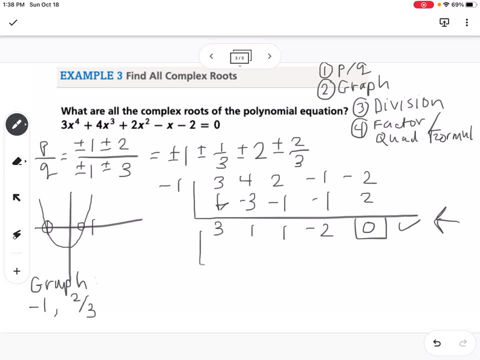 can keep going from there So we can get it simpler and simpler, simpler. So now I'm going to check 2 thirds. So 3 times 2 thirds would be 2, so it would be 3,, 2,, 3, 2, and this one also worked. So now what's left over here is we have 3x squared. 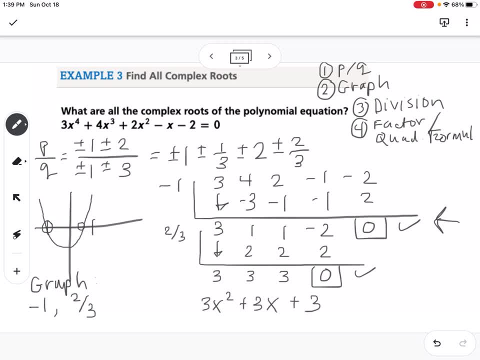 plus 3x plus 3.. So we can factor 3 out of all of that, so we can set that equal to 0, so we can divide by 3, so that would be x squared plus x plus 1 equals 0. And now we're. 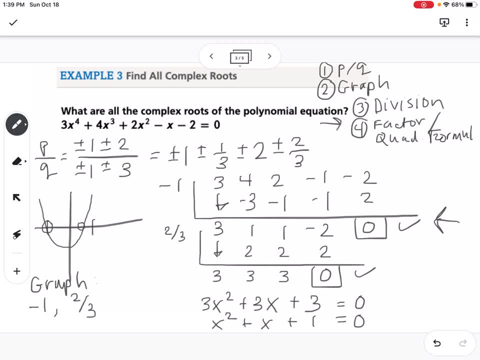 at that step 4.. So we've tested both of the possible rational zeros. so that means that our remaining zeros would either be irrational- which from the graph it didn't look that way because it doesn't look like it's crossing another point- or they could be complex. So 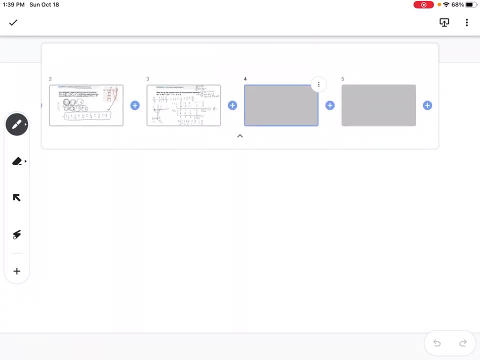 now what we would do. let's Okay, so I'm going to keep going with this. So we had x squared plus 3x, nope, plus x plus 1.. So if I use the quadratic formula, this would be negative: 1 plus or minus square. 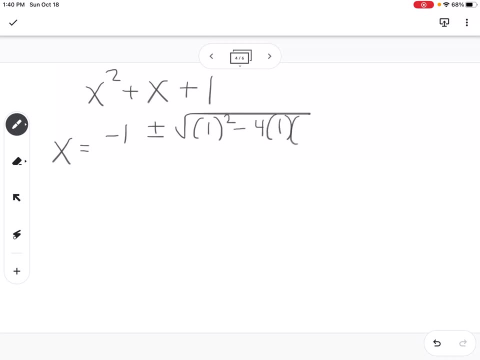 root of 1 squared minus 4 times 1 times 1 over 2 times 1.. So this would be 1 minus 4, so it would be negative 3 over 2.. So that means my two complex solutions would be negative: 1 half plus or minus square root of 3 over 2i. So all my 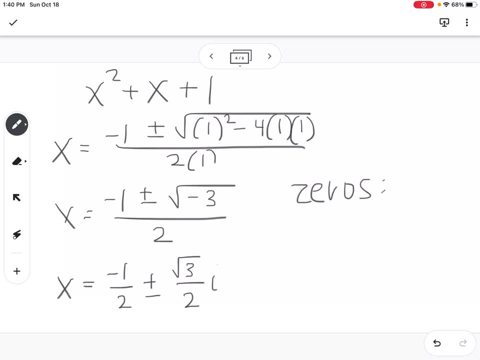 zeros wereso it was negative 1, 2 thirds and then negative 1 half plus or minus square root of 3 over 2i. So again, these are real and these are complex. So the other thing is, when we're finding all 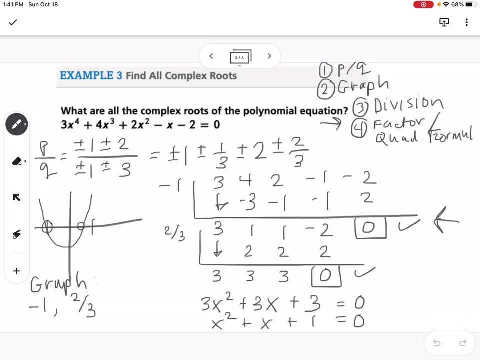 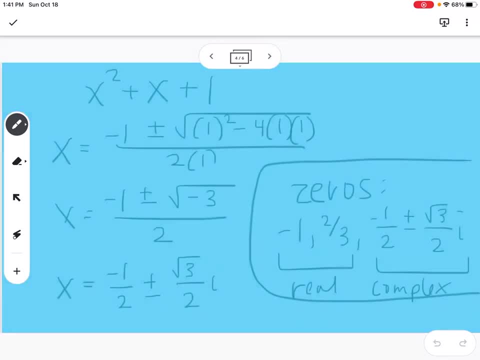 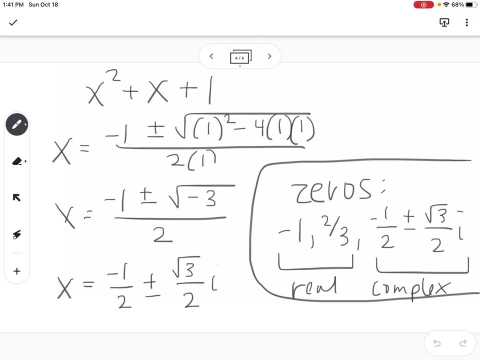 of the zeros. the degree of our polynomial tells us how many total zeros we should have. So this was a fourth degree polynomial and you can check. we have four different solutions, four different roots, four different zeros. So that matches Okay. 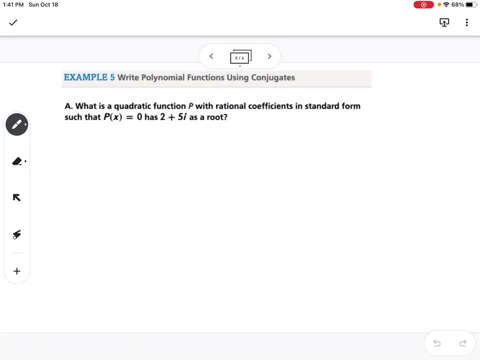 Example 5.. Example 5 says: write a polynomial function using conjugates. What is a quadratic function? p with rational coefficients in standard form, such that p of x equals 0 has 2 plus 5i as a root. So something you need to know about complex numbers is that if you have one complex number, 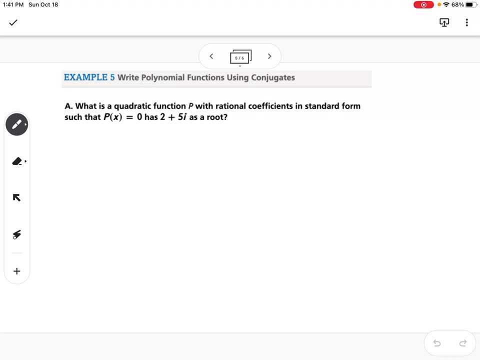 that is a root of your polynomial, then that means its conjugate also has to be a root of your polynomial. So that means that 2 minus 5i Is also a solution. So if we take this, so p of x equals: 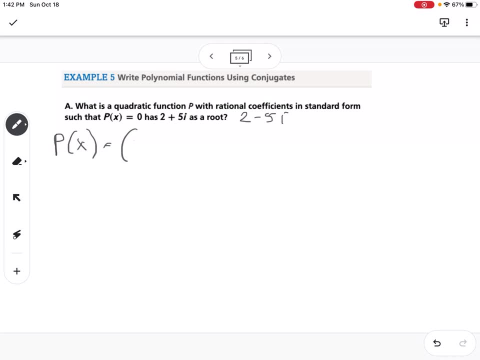 So when we take our solution, so we would write it as a factor. So this would be x minus 2 plus 5i And x minus 2 plus 5i. So then, if we get rid of the parentheses, distribute the minus, we would have x minus. 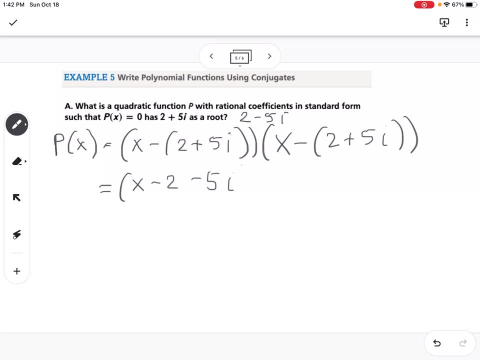 2 minus 5i, 5i and x minus 2 minus 5i. Wait, I wrote plus for both of these, Oops, So that would be plus 5i. There we go, Okay. so now I can group these first two terms and what you. 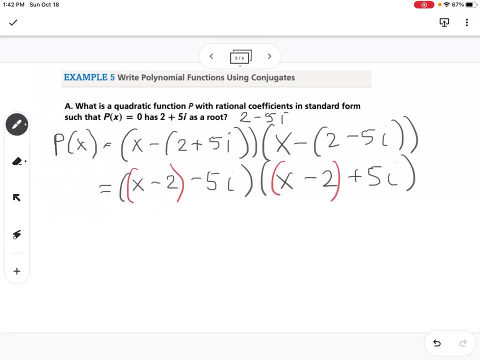 hopefully will notice, is I have two conjugates that are being multiplied by each other now, So I have x minus 2, and so if we FOIL this out, as the x minus 2 is one term and the 5i is the second term, if we FOIL this out, the middle terms will cancel. So what I'll end? 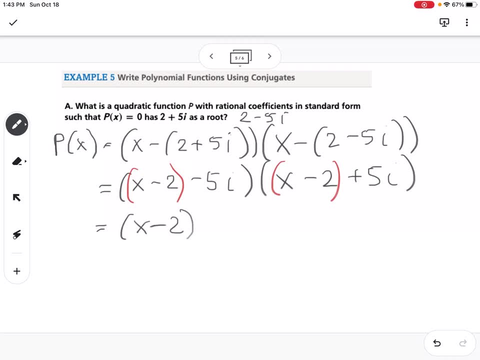 up with is x minus 2 squared minus 25i squared, So the middle terms, the x minus 2 times 5i and times negative 5i, those will cancel. So then what this would be is x squared minus 4x plus 4, if I FOIL that out And then remember, 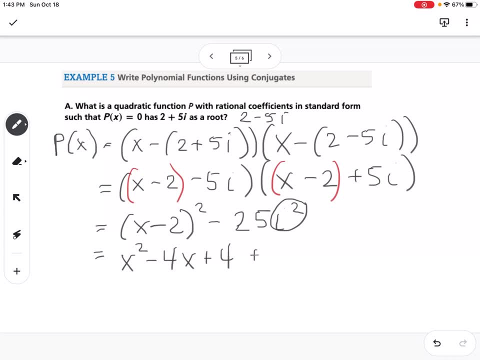 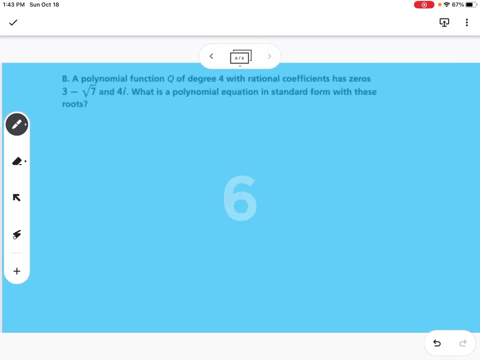 i squared is negative 1, so this would turn into plus 25.. So my final polynomial here would be x squared minus 4x plus 29.. Okay, part b of this says a polynomial function q of degrees. So right here, that tables the degree, with 4i squared minus 5i squared, So we have 1, 0, with rational coefficients has 0s, 3 minus square root of 7, and 4i. So, just like with complex 0s, if you will have 1, 0, that means that we have to have the conjugate.